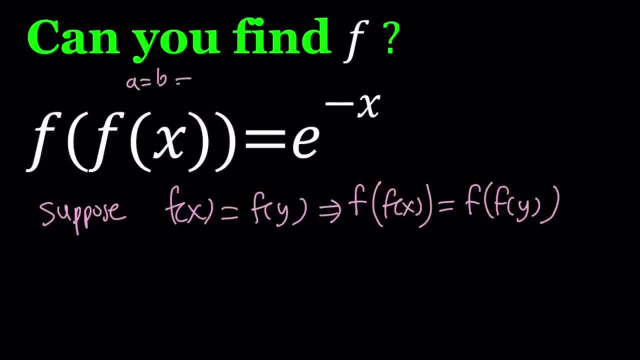 defined for functions. if a is equal to b, then f of a is equal to f of b. Obviously, right. you can have different outputs for the same exact same input. Okay, now we do know something about f of f of x. right, it's given as e to the power negative x, and f of f of y is just the same equation. 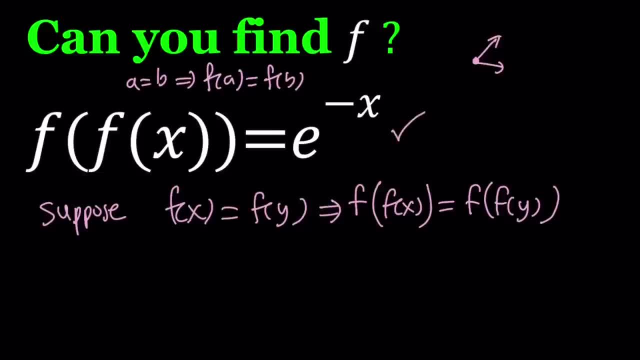 where x is replaced by f of f of y. So we're going to take f of f of x and we're going to replace with y. So f of f of x is e to the power negative x and f of f of y is just a replacement. 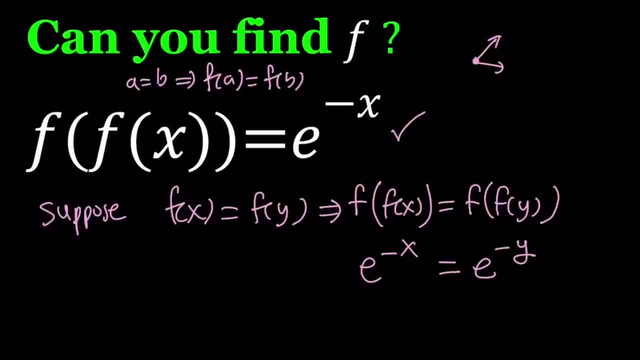 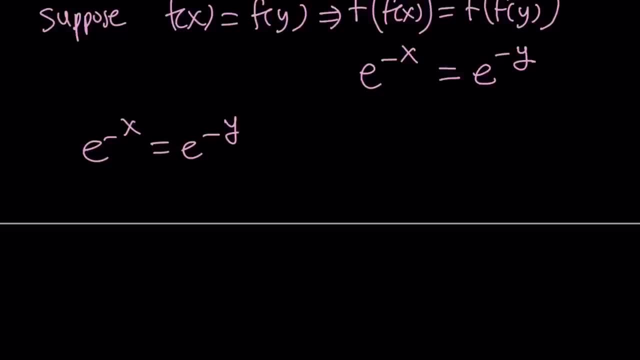 of x with y and it is e to the power negative y. Great. and what does this imply? If e to the power negative x equals e to the power negative y, then this just implies that negative x equals negative y, and that implies x equals y- Awesome, Great. and where does this come from? It basically follows: 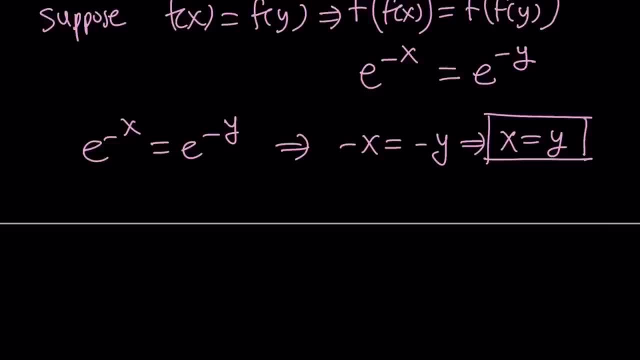 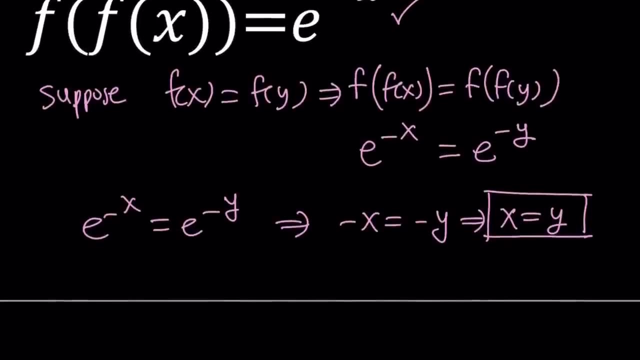 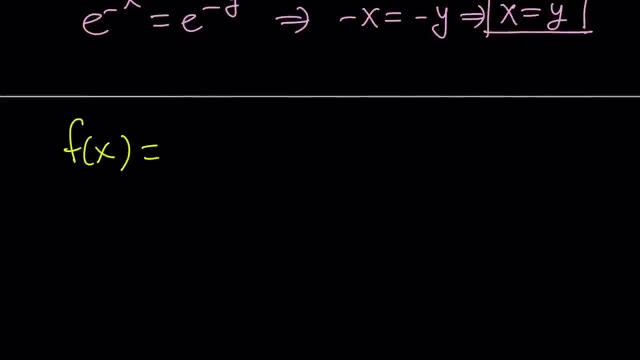 the fact that e to the power x is always increasing and it is basically one to one. Okay, so x equals y follows from the initial assumption, which is f of x equals f of y. So let's go ahead and put those together. F of x equals f of y implies x equals y. Notice that this is not always true for all. 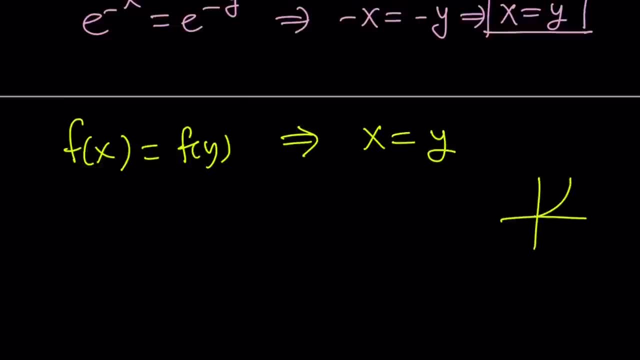 functions. For example, if you think about y equals x squared to the parabola, then you may have the same f of something value, but that doesn't mean the inputs are equal. They could be the opposites, right. So in other words, if you have f of x equals x squared, then x squared equals. 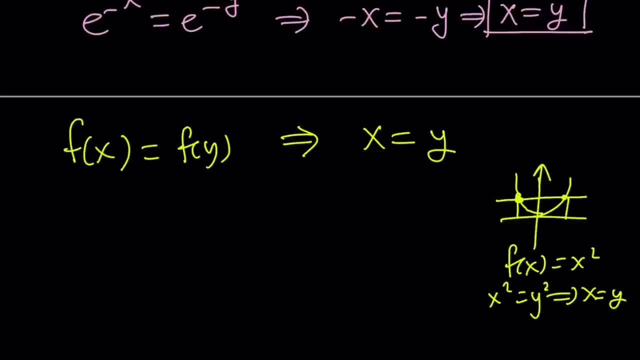 y squared doesn't always imply x equals y, because it could also imply x equals negative y. Make sense? Okay, great. but so this is a very special condition, and this means that f is one to one. You could also call it an injection, or you could say: 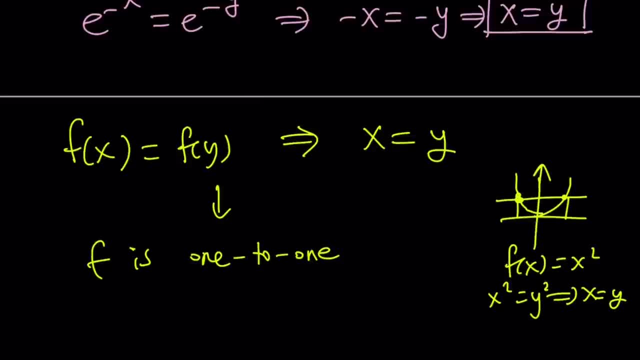 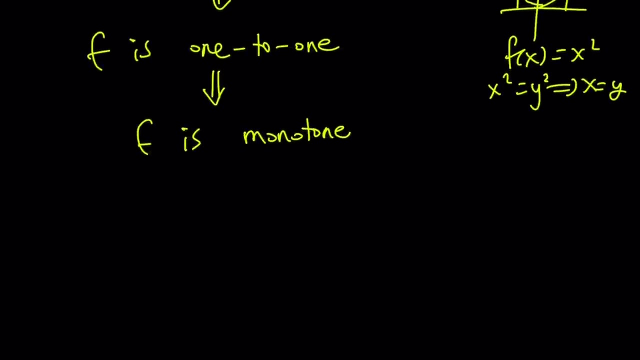 f is injective. Okay, since f is one to one, this basically means that f is monotone. What does monotone mean? It's either monotonically increasing or monotonically decreasing, So we're going to look at both cases and see what happens. Okay, again, our goal is to 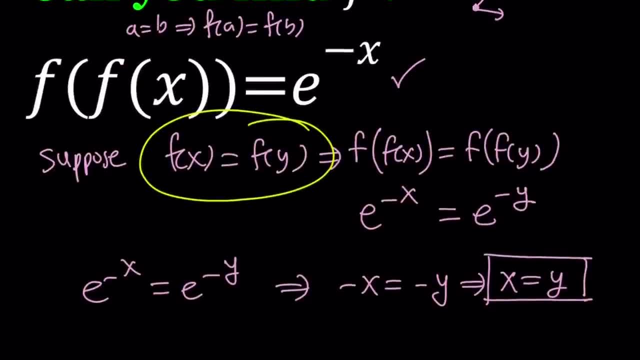 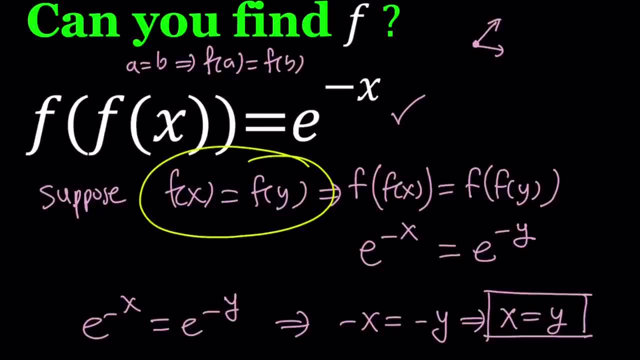 find a function whose composition with itself is e to the power, negative x. Obviously, at this point you can speculate about f of x. What could it look like? Is it e to the power? something Is it? does it contain ln or some other things? That's definitely going to help. 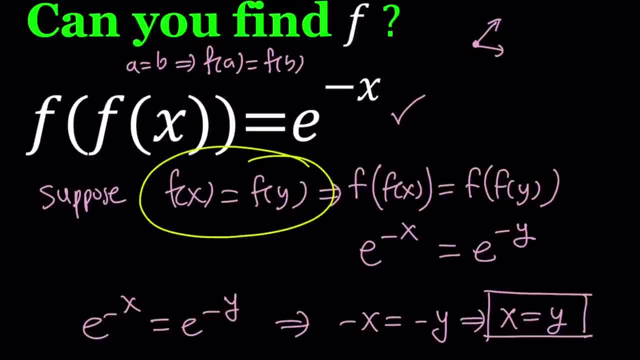 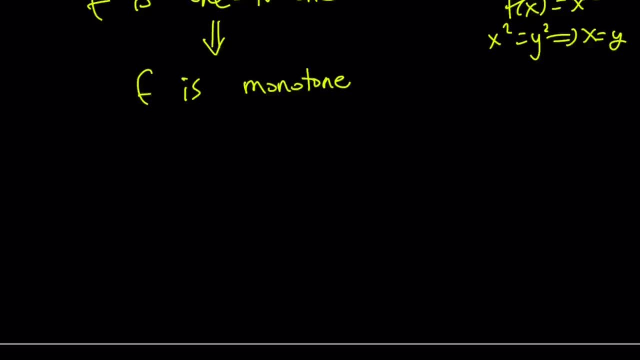 you, you know, to see a little deeper into the problem. Anyways, so f is monotone because it is one to one. Okay, so if so, let's go ahead and look at two cases. First case: if f is monotonically increasing. Monotonically increasing basically means that it preserves the order. So 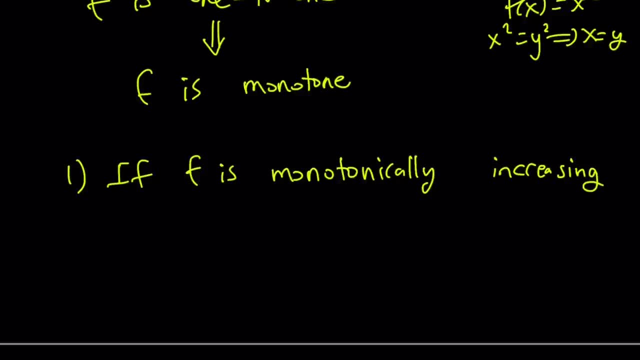 if you have a input that is greater than another input, then their outputs are also going to be in the same order. Make sense? In other words, if x is less than y, then this implies f of x is less than f of y. That's what monotonically increasing means. Obviously, you could also write this for x. 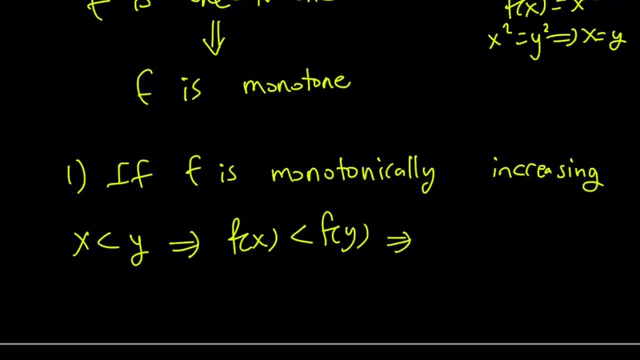 is greater than y, but it's not going to be greater than y. So if you have an input that is greater than y, then it's going to be the same thing. Now let's go ahead and apply f on both sides. And since f is 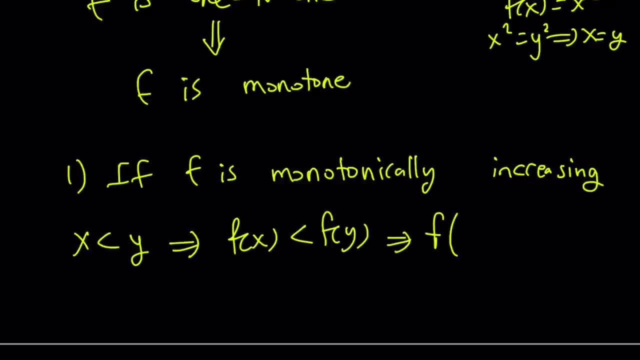 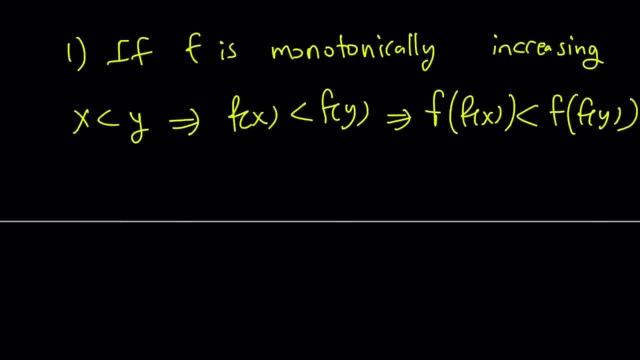 monotonically increasing. the order is not going to change. So f of something is going to be less than f of the other thing. Because they are arranged that way, Make sense, Cool. But we do know what f of f of x is right. So the whole idea is to bring it to the composition field so that 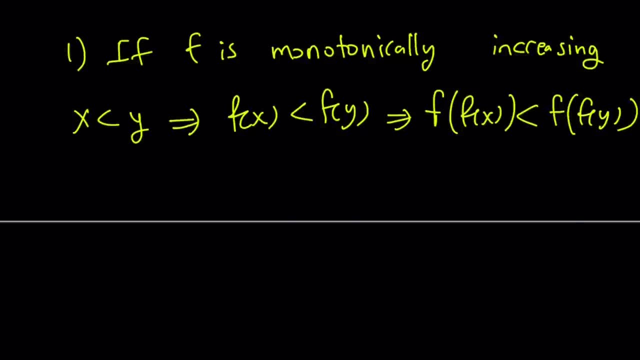 we can replace it with something And this means that e to the power negative x is less than e to the power negative y And obviously when you reverse the process- e to the power negative x and e to the power negative y- cannot be negative or zero. So we can easily say that this is one over e to the x and 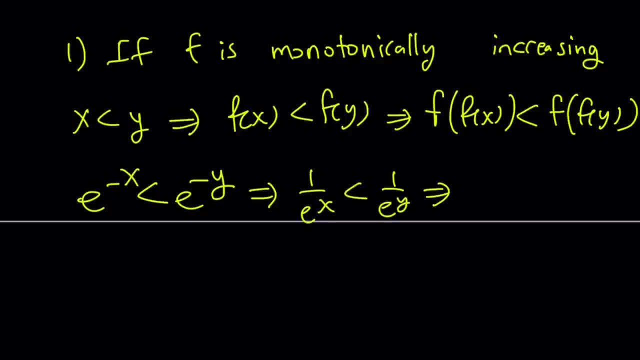 this is one over e to the y, And when you take the reciprocals the order will be reversed, which means e to the power x will be greater than e to the power y And, as you know, e to the power x as a function is monotonically increasing. We can use the same term here, And this implies that 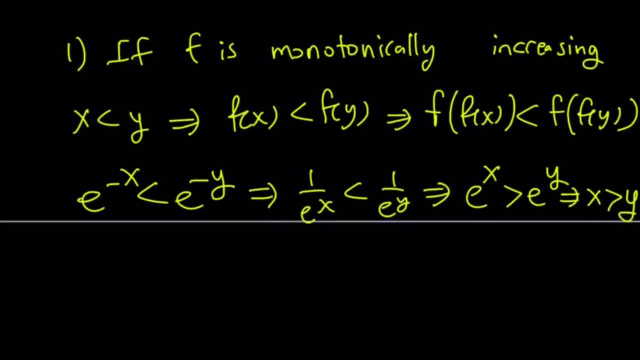 x is greater than y. Okay, great. So what did we start with? We started with: x is less than y. That's the assumption, Or I could say the assumption was that f is monotonically increasing, which implies that, by the way, And we arrived at a contradiction, Because if x is less than y, it can't be greater. 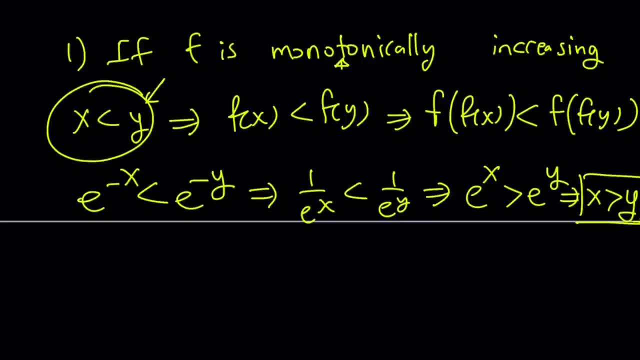 than y Make sense. So this is a contradiction which means f cannot be monotonically increasing. So we are left with the second option Right, Which is, if f is monotonically decreasing, All right, Awesome Now. so here's what we're going to. 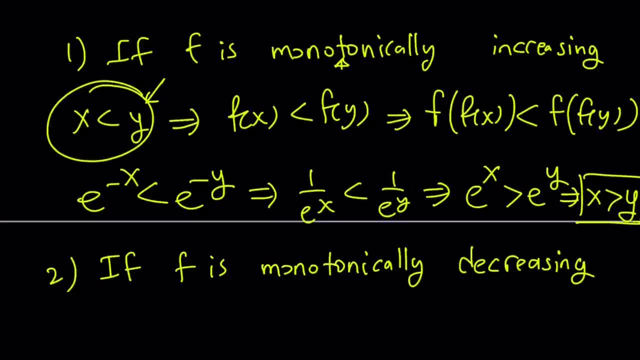 do Monotonically. increasing means you have a function like e to the power x, where you take two input values. One is less than the other. Let's say the smaller one is a, The larger one is b And when you look at f of a and f of b, you're going to see that f is less than the other. 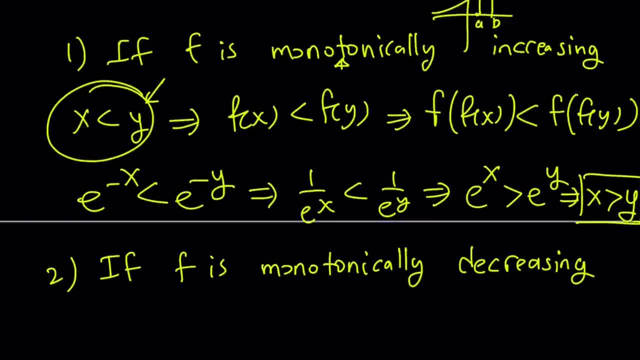 But I noticed that because b is greater than a, f of b is also greater than f of a. So when you apply f on both sides, the order of the inequality or the sign does not change. Make sense With the monotonically decreasing And I can give you an example of a monotonically 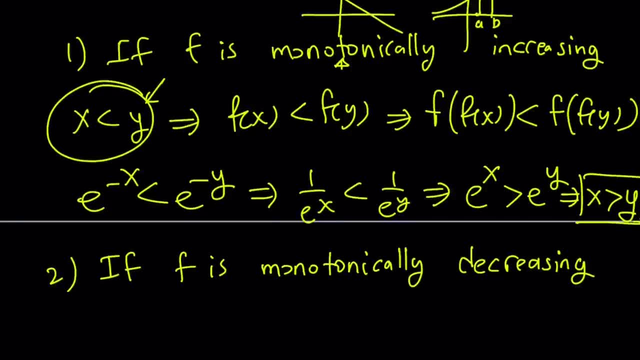 decreasing function, such as something like y equals negative x plus one, This will be monotonically decreasing. So when you pick two values- Let's say b is greater than a And it's Output is going to be less than the output of a- Make sense. So in other words, if f is 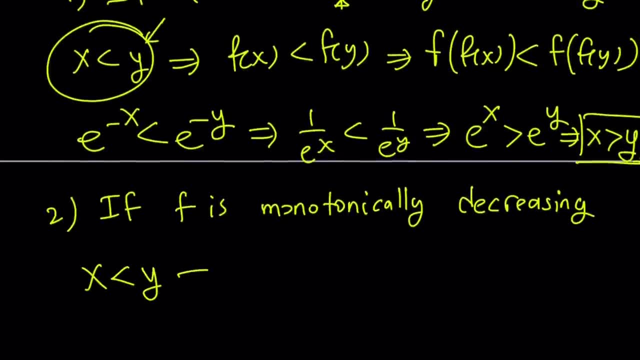 monotonically decreasing x is less than y is going to imply f of x is greater than f of y. Notice that the order changes Make sense And when we apply one more time, obviously the order is going to change again. This is the critical part. So f of f of x is going to be less. 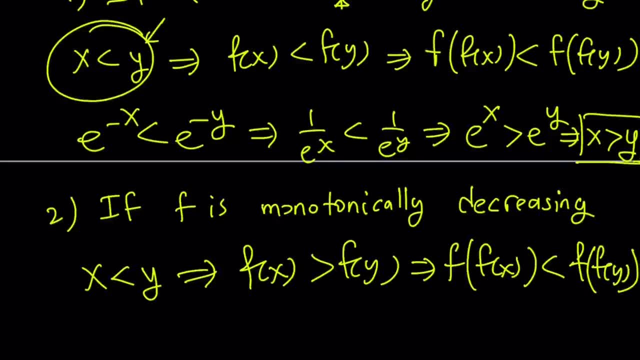 than f of f of y, because f of x is greater than f of y, Make sense. Notice that the order of f of x and the order of the inequality changes every time you apply f, But this means f of f of x is less. 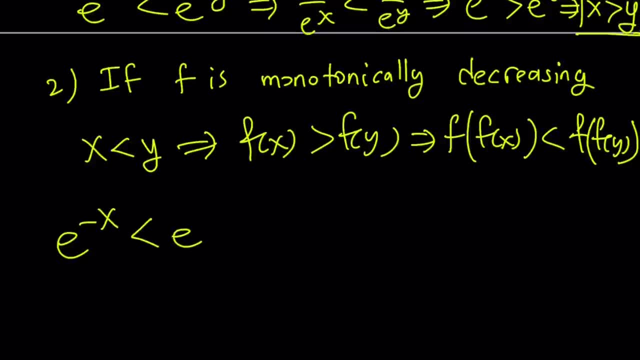 than f of f of y means e to the power negative x is less than e to the power negative y. And again this means 1 over e to the x is less than 1 over e to the y. Again, e to the x and e to the y are. 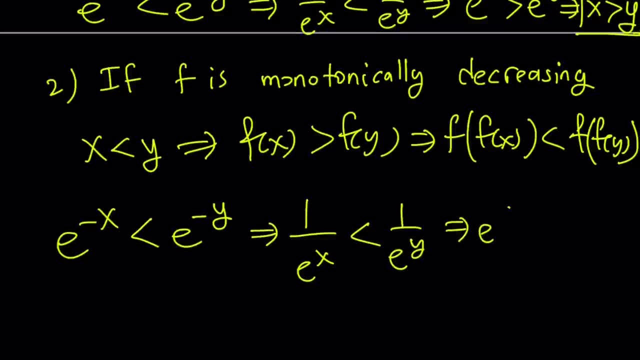 always positive, And this would imply e to the power x is greater than e to the power y. And since e to the power x is a function is monotonically increasing, it will preserve the order. This will imply x is greater than y, And again we arrive at a contradiction, Right, Which means: